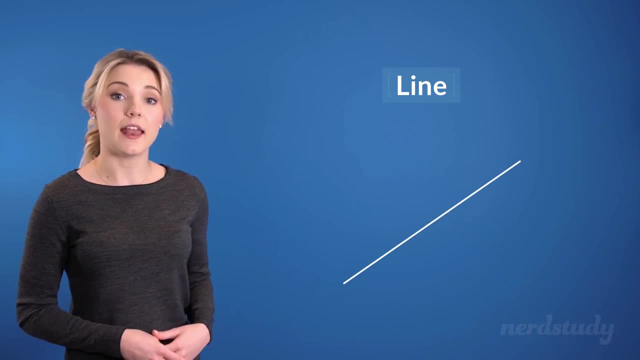 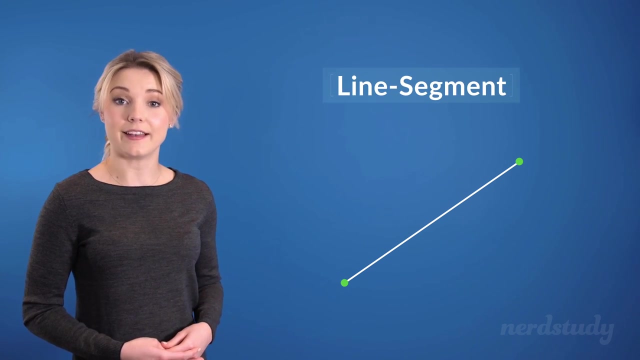 line is defined as being straight, with no curves and never ending on either sides. However, if the line was not never ending, but instead had two specific endpoints, like so, then we would not call this a line anymore. Instead, we would call this a line segment. 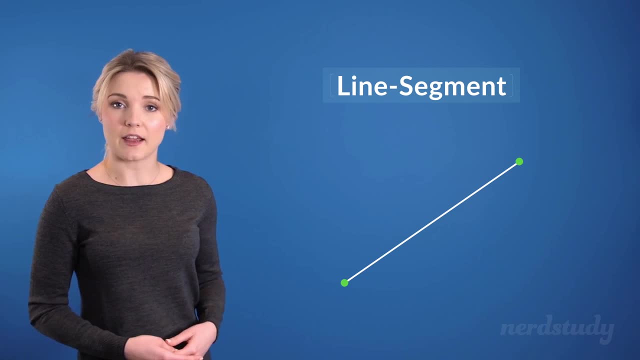 Awesome. Now I want to stress that a line segment is similar to a line, only that both sides of the line has endpoints. However, if only one side had an endpoint and the other extended to infinity, we would call that a ray instead. Now lines, rays or line segments can come together to form something. 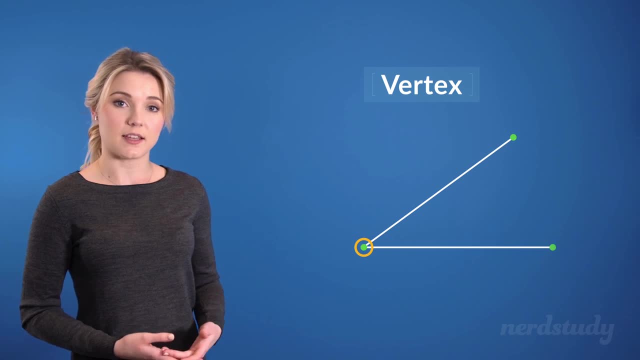 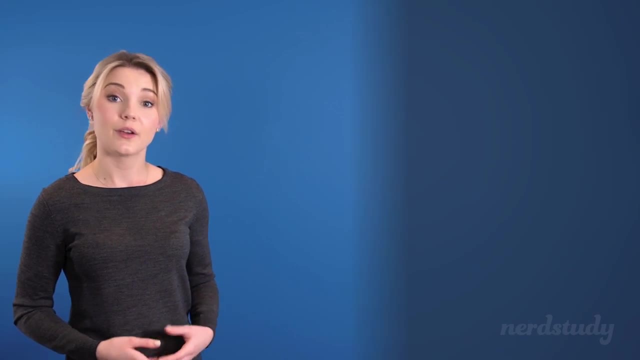 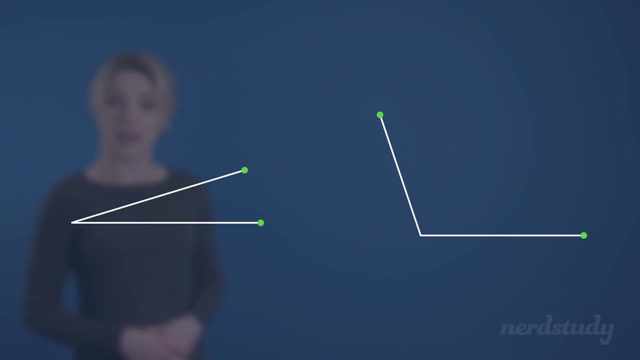 called a vertex. In this case, as we can see, we've got two line segments that come together at this point, or shall I say this vertex Cool. So now I want us to take a look at another example of a line segment. 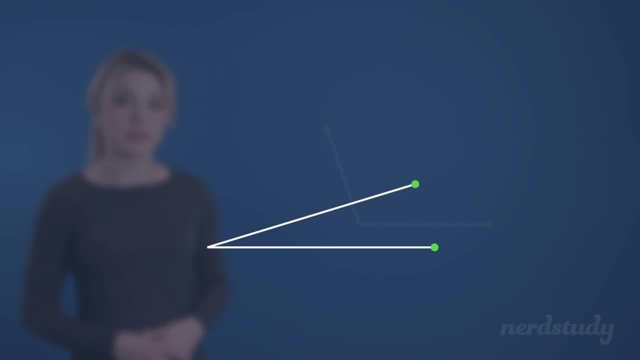 Now, let's say that we have two line segments coming together. Notice how these line segments come very close to each other, while these ones come together very far apart from each other. Well, we can actually measure the distance of each of these with what we call. 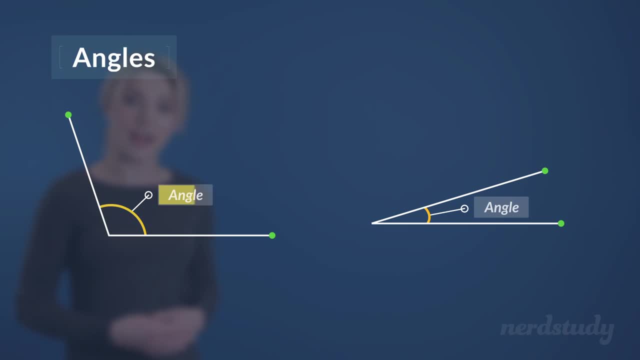 angles. Now, clearly, this angle here is greater than this angle. So I'm sure we've all heard the expression rotating 360 degrees, but this expression actually applies for many other math as well. To have an angle of 360 degrees is exactly one full circular rotation, where 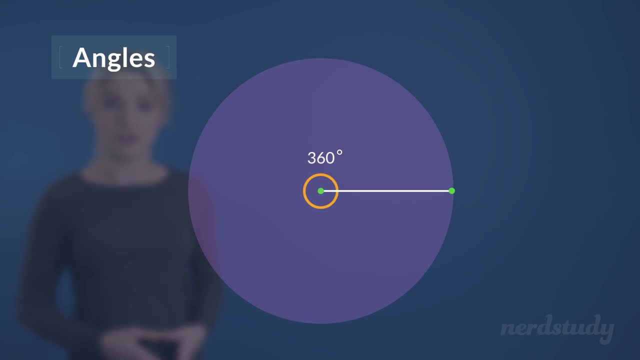 each degree accounts for a certain amount of angling rotation And instead, if we were looking at half of 360 degrees, which would be 180 degrees, we would be looking at half of the rotation of a circle And, of course, what we end up with is the two line segments. 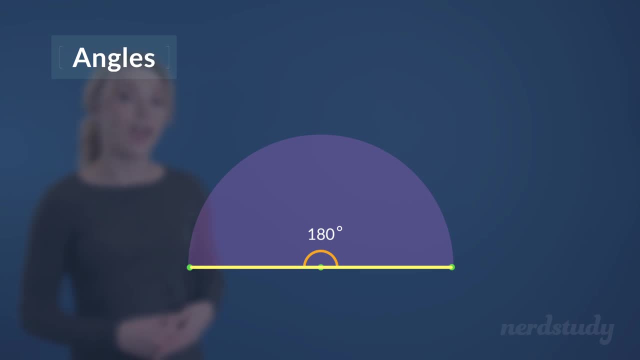 creating just one flat line segment And, naturally, half of 180 degrees is 90 degrees for an angle that looks like this, which is actually quite special, as we will learn in the near future. Therefore, we have a special way to show this angle, and it is by drawing in these two little lines in order.